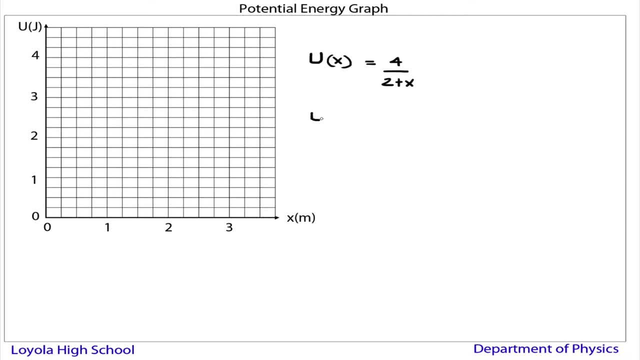 So we've seen this is a little unfamiliar. we've seen an equation that looks like this: So u equals 1 half kx squared for a spring. so it's a spring system. So this is something a little bit different. 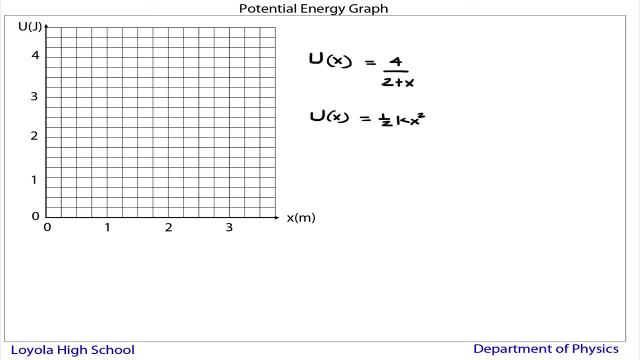 Not sure what this system is- maybe a ball on a wrap or a different type of spring- but we do know the potential energy equation for it. So let's stick with this one right here and let's take a look at what the graph looks like. 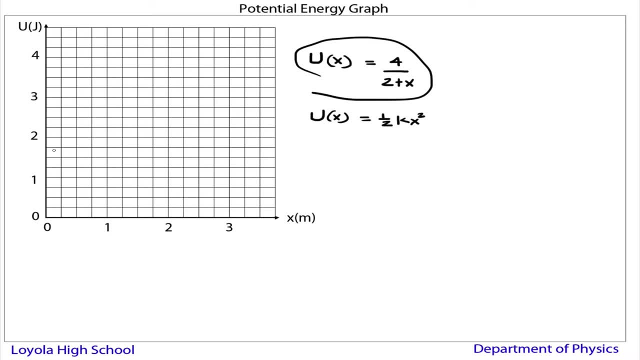 So let's see: when x is 0,, let's graph it. when x is 0,, we get the value of 2.. When x is 1,, we get 4 thirds. So let's see: x is 1,, no more than. 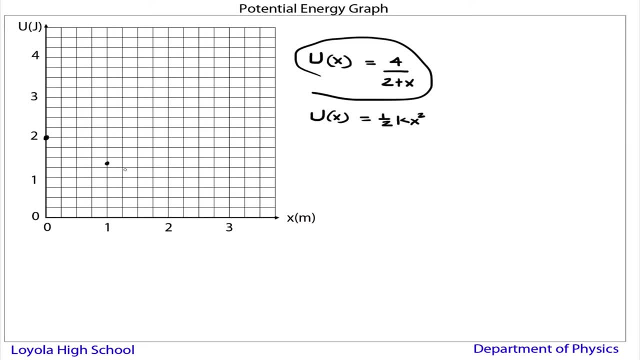 Right around here. I think it is: When x is 2, we get the value of 1.. And when that value is 3, we get 4 fifths- a little bit less than 1.. Okay, So we get something that looks like it's a 1 over x type function that decreases here like this: 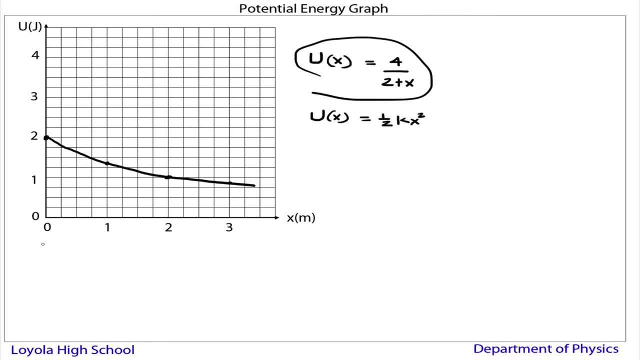 Alright. So the question is this: For whatever this system is, we're going to find. We're going to find if the velocity at 0 equals 0, so if it starts from rest. so at this point, right here, if the velocity is 0, 0, we want to find the velocity when x is equal to 2.. 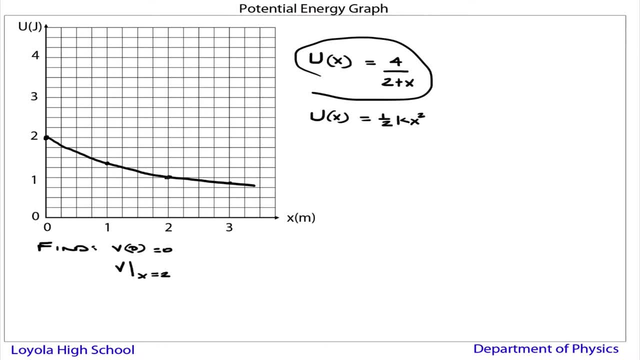 So when this object does get to this point- value of 2, how fast is it going? So solution: So this is a conservation of energy type problem. So what we're going to say is: we know some information here at point 2, so I'm going to draw two buckets here. 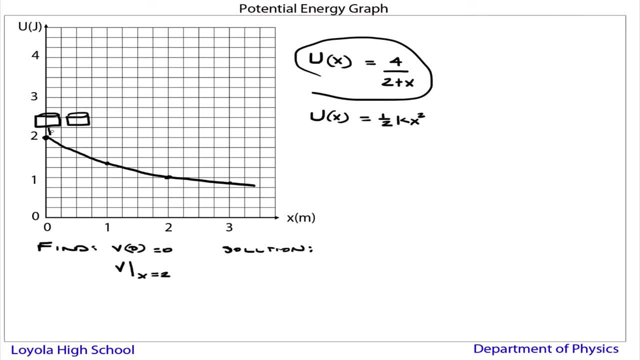 I'm going to draw a kinetic energy bucket and a potential energy bucket. Now, normally I would do a gravitational and elastic, but I'm not sure what types of potential it is. I just know the total is a value of 2 at this point. 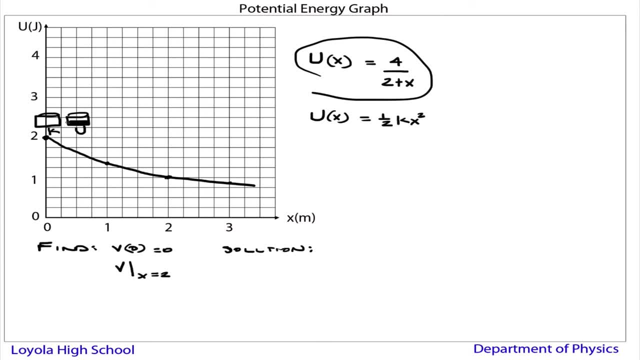 So I'm not going to differentiate between Between gravitational and elastic, It's just, the total is 2 there And over here, and we have no kinetic because it starts from rest. And at this point here I'm going to draw two more buckets.